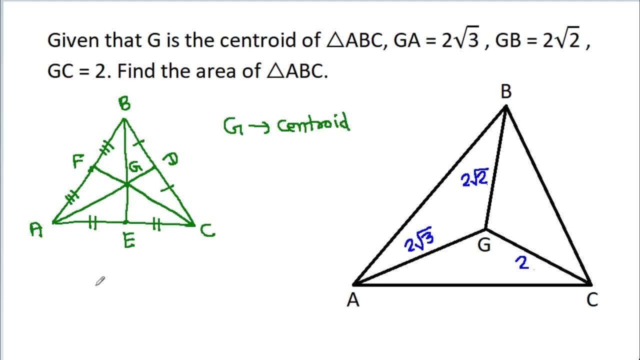 and also AG ratio GD, it will be 2 ratio 1, and BG ratio GE, it will be also 2 ratio 1, and CG ratio GF, it will be also 2 ratio 1, and also these 6 areas. they will be equal. 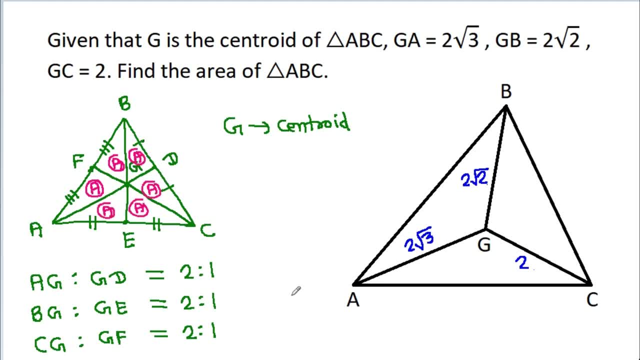 Suppose A. so here, area of AGB, it will be equal to area of BGC, it will be equal to area of AGC. that will be A plus A, that is 2A. So these three areas, they will be equal. 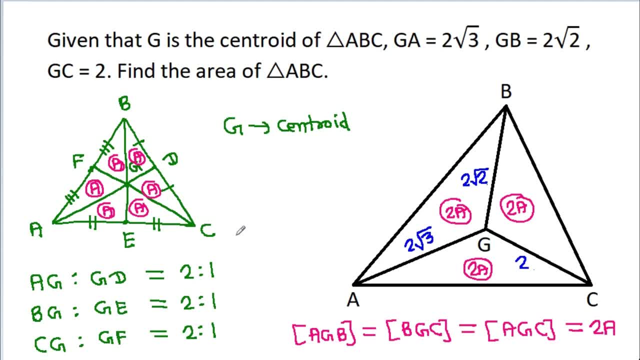 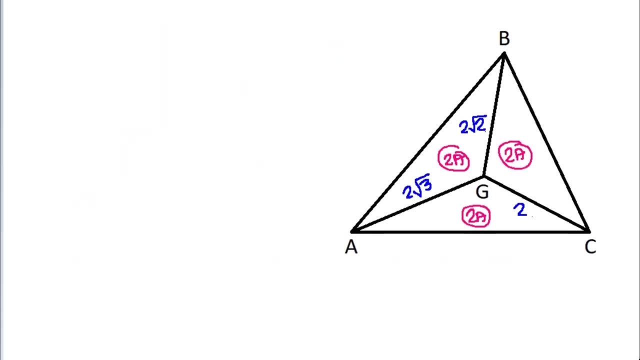 And A plus A, that is 2A. So these three areas, they will be equal. And So these three areas, they will be equal, And now. So these three areas, they will be equal, And now. So these three areas, they will be equal, And now. 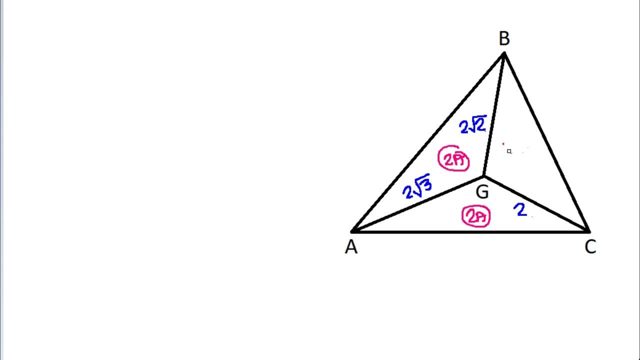 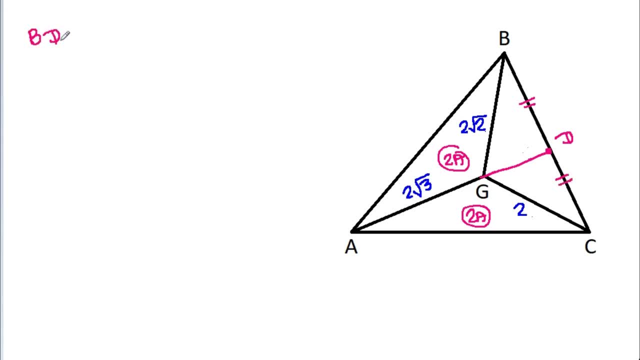 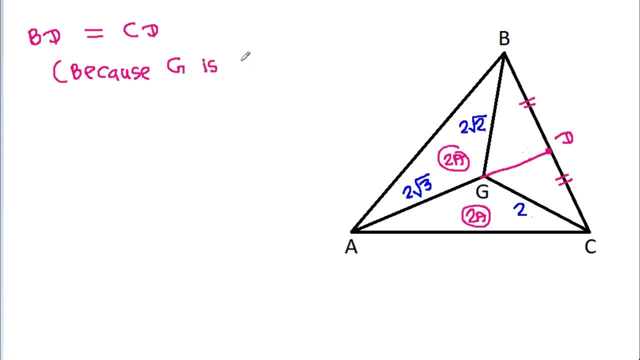 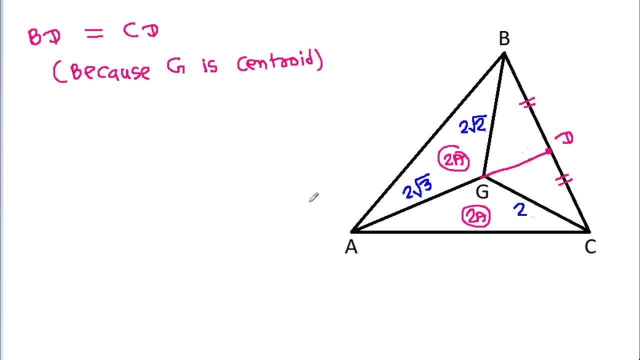 here, if we extend AG And if we extend GD, to suppose E such that AG it is equal to GE- It is our construction- Then we know that AG ratio GD it will be equal to 2 ratio 1.. 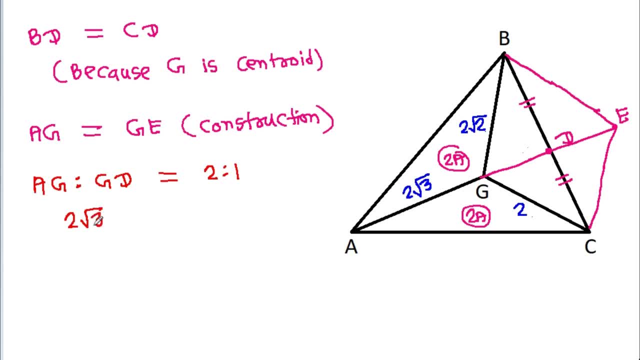 And AG is 2 times a square root of 3. by GD, it is equal to 2. by 1. And 2 will be equal to 1.. So, GD, it will be equal to a square root of 3.. 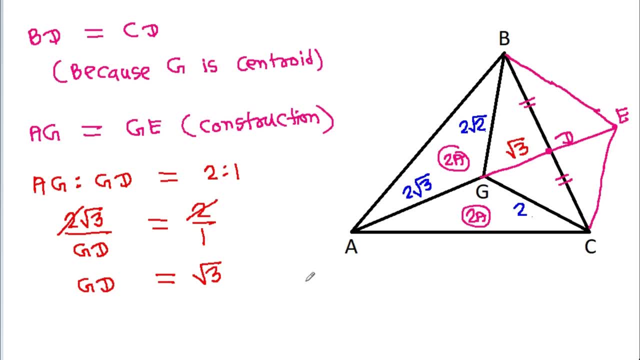 GD. it is a square root of 3.. And we have: AG is equal to GE And AG is 2 times a square root of 3.. It is equal to GE. So GD is a square root of 3 minus DE. 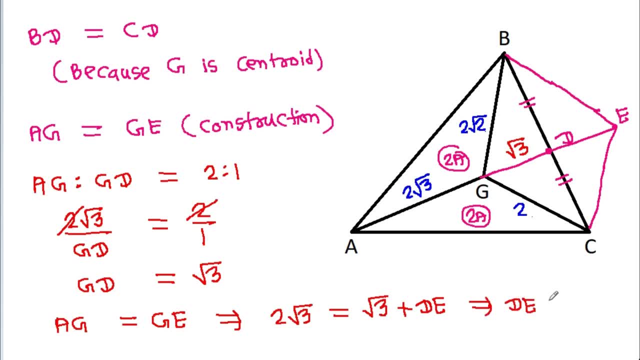 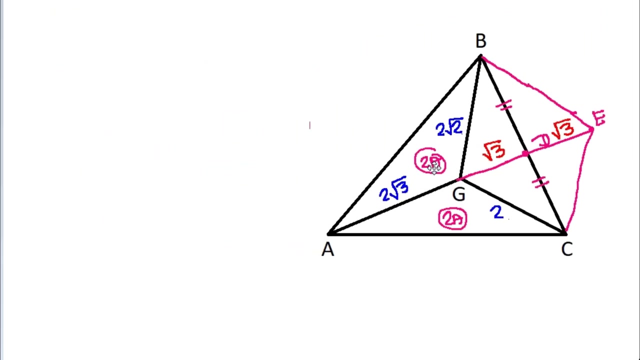 That means DE. it will be equal to a square root of 3. DE it will be a square root of 3. And, and, and, and. it is our construction Now in BGCE. It is BGCE. 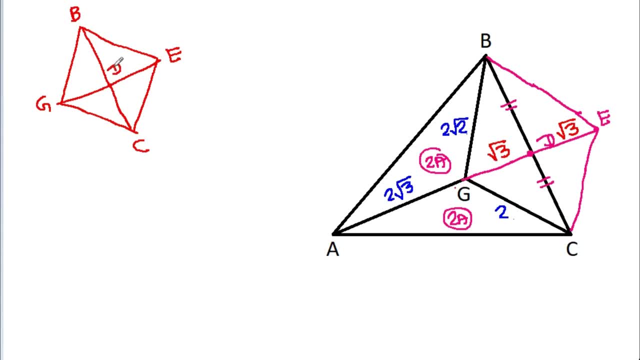 This point is DE And We have: GD is equal to DE. that is a square root of 3, GD it is equal to DE and BD it is equal to CD, BD it is equal to CD. So digolons bisect each other. that means BGCE. it will be parallelogram. 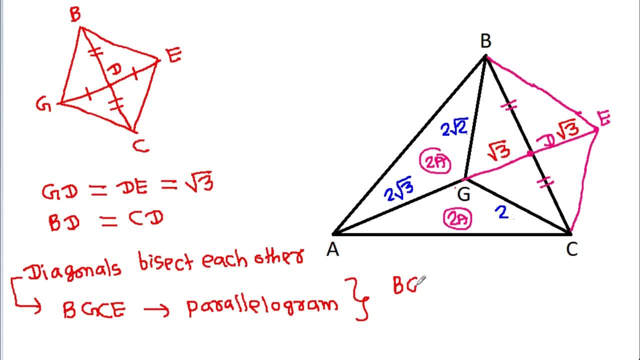 Hence BG it will be parallelogram, It will be equal to CE and BE it will be equal to GC. So CE it will be also 2 times a square root of 2, and BE it will be 2.. 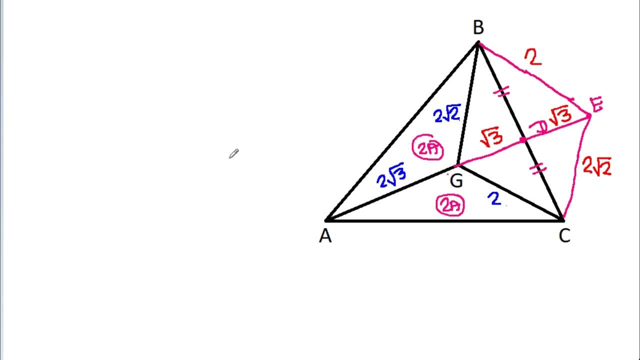 Now interangle BGE. we have: GE square is equal to 2 times a square root of 3, a square that is 2N and BGS square plus BE. So GE square it is equal to 2 times a square root of 2, a square plus 2, a square that 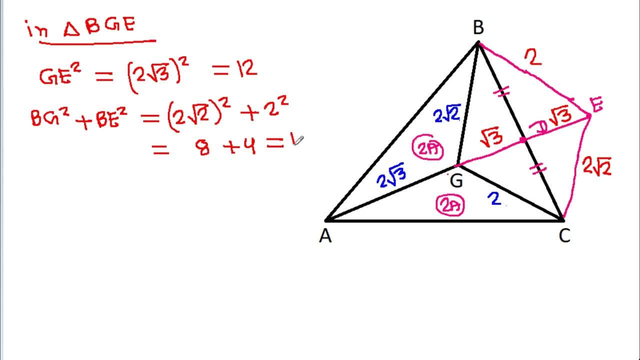 is equal to 8 plus 4, and it is 12.. So GE square: it is equal to BGS square plus BE square. That means angle GBE square. So GE square: it is equal to 2 times a square root of 2, a square plus 2A square. that is equal to 8 plus 4, and it is 12.. 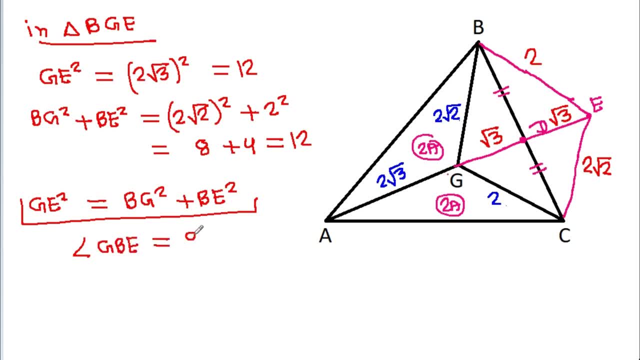 So GE square it is equal to BGS square plus BE square it will be equal to 90 degree. this angle it will be 90 degree. and now we know that BGCE it is parallelogram and angle GBE it is equal to 90 degree. that means BGCE it will be rectangle. 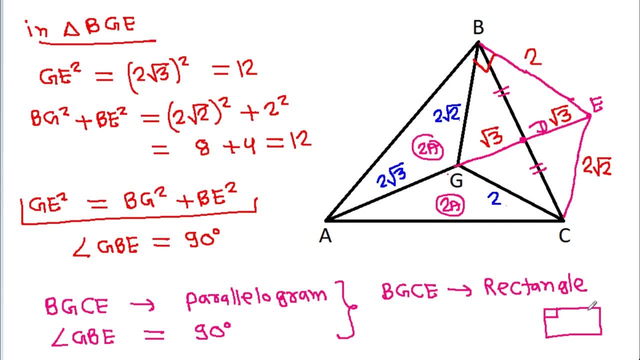 and in any rectangle all the angles are 90 degree and in any rectangle, all the angles are 90 degree and in any rectangle all the angles are 90 degree. so angle BGCE, it will be also 90 degree, this angle, it will be 90 degree, and 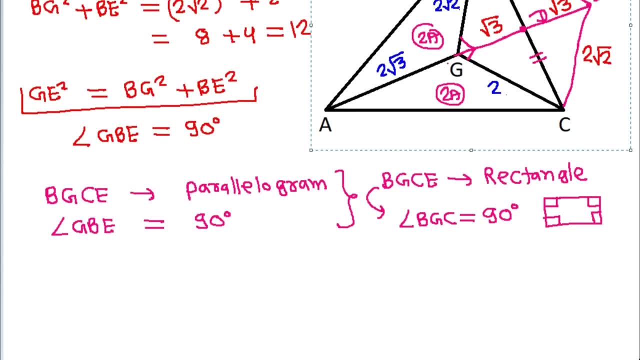 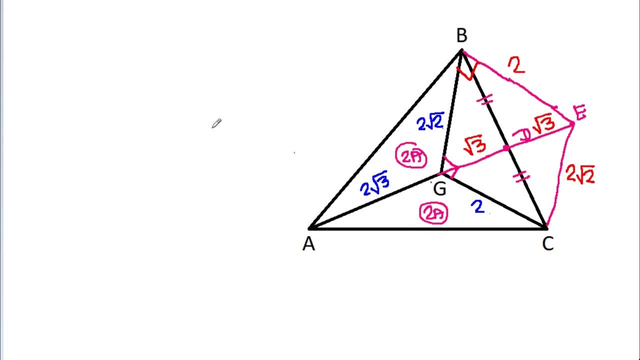 and now interangle, interangle, interangle, BGC. It is BGC. This angle is 90 degree. BG is 2 times s square root of 2.. GC is 2.. So area of BGC it will be equal to 1 by 2 times base is 2 times height is 2 times s square root of 2.. And 2 will 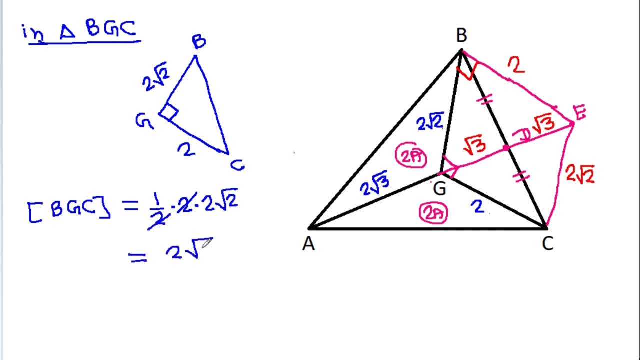 get cancelled. So it is 2 times s square root of 2.. And we have: area of AGB is equal to area of BGC is equal to area of BGC. So area of BGC is equal to area of BGC. So area of BGC is equal to area. 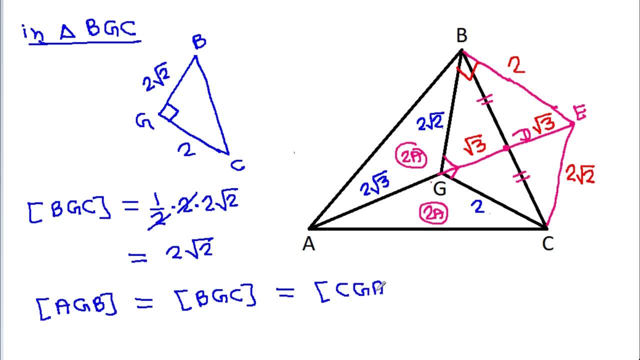 of BGC is equal to area of CGA, So it will be equal to 2 times s square root of 2.. So area of ABC, it will be equal to area of AGB plus area of BGC, plus area of CGA.